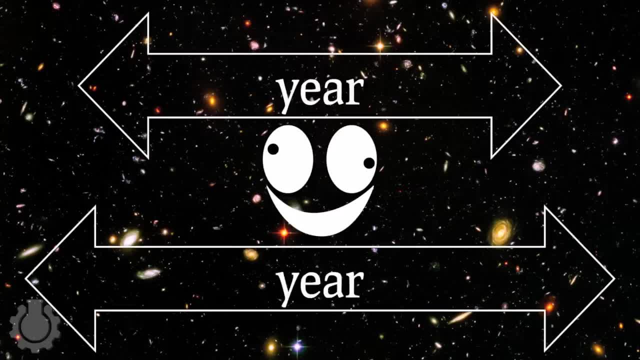 Why does that happen? What kind of crazy universe do we live in, where some years are longer than others? To answer this, we need to know just what is a year. Way oversimplifying it, a year is the time it takes the earth to make one trip around. 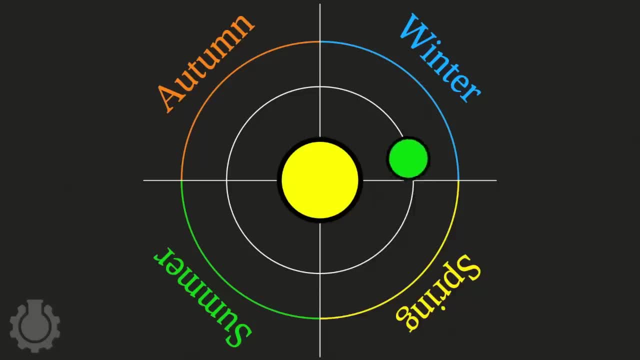 the sun. This happens to line up with the cycle of the seasons. Now, drawing a little diagram like this, showing the earth jauntily going around the sun, is easy to do, but accurately tracking a year is tricky when you're on earth, because the 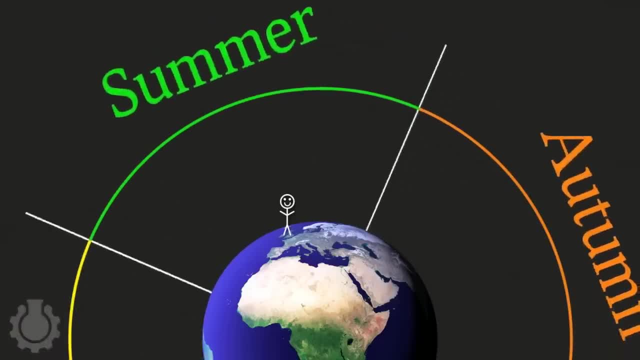 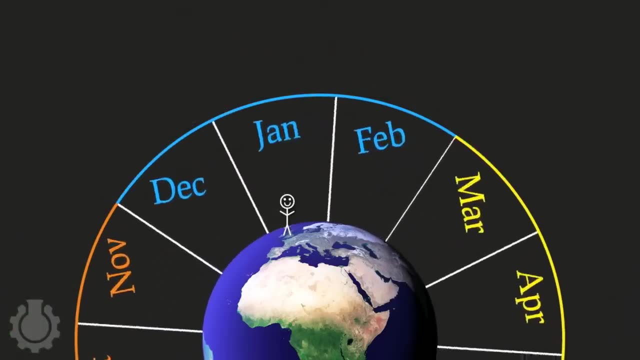 universe doesn't provide an overhead map. On earth. you only get to see the seasons change and the obvious way to keep track of their comings and goings is to count the days passing, which gives you a 365 day calendar. But as soon as you start to use that calendar, it 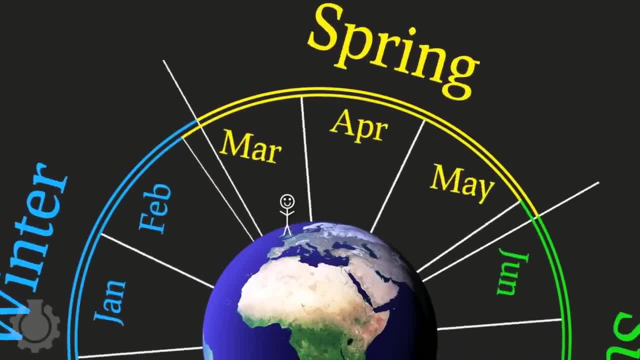 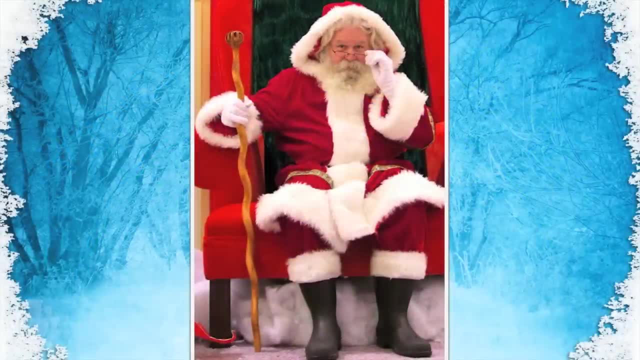 slowly gets out of sync with the seasons, and with each passing year the gap gets bigger and bigger and bigger. In three decades, the calendar will be off by a week, and in a few hundred years the seasons would be flipped, meaning Christmas celebrations taking place. 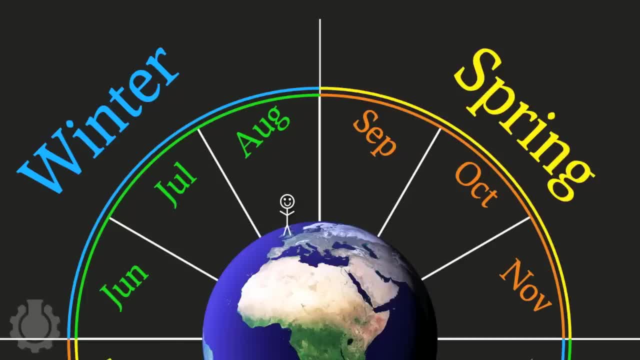 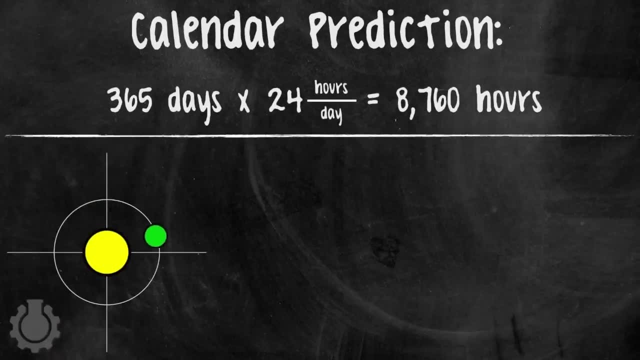 in summer, Which would be crazy. Why does this happen? Did we count the days wrong? Well, the calendar predicts that the time it takes for the earth to go around the sun is 8760 hours, but if you actually timed it with a stopwatch, you'd see that a year is really. 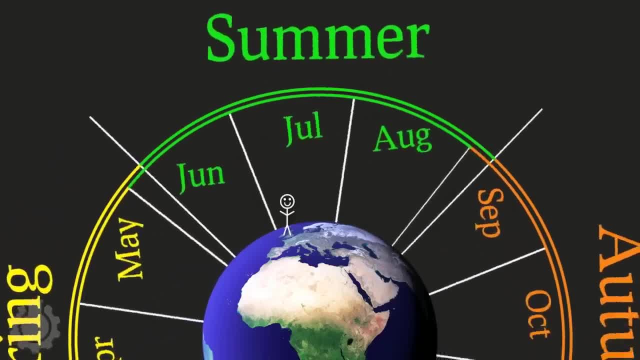 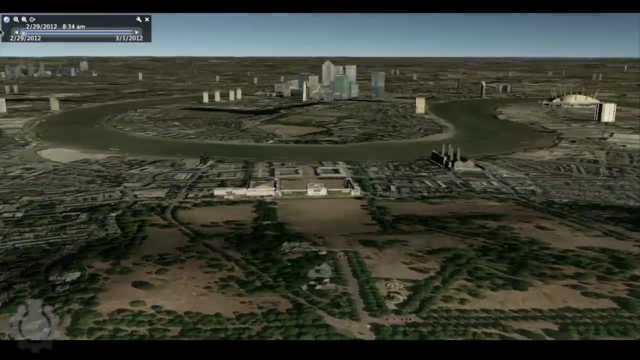 longer than the calendar predicts, by almost 6 hours. so our calendar is moving ever so slightly faster than the seasons actually change, And thus we come to the fundamental problem of all calendars. the day-night cycle, while easy to count, has nothing to do with the yearly cycle. Day and night are caused by 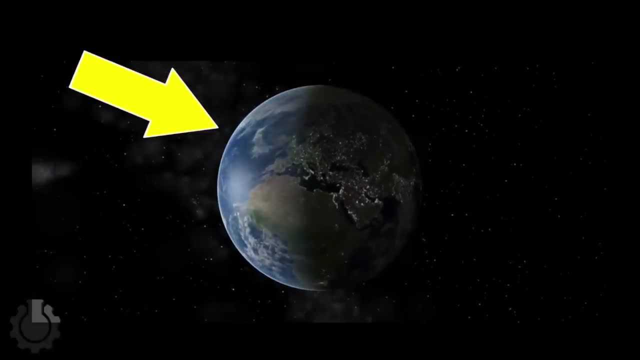 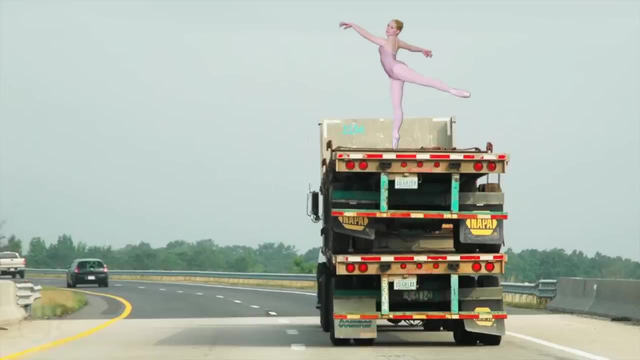 earth rotating about its axis. when you're on the side facing the sun, it's daytime and when you're on the other side it's night. But this rotation is no more connected to the orbital motion around the sun than a ballerina spinning on the back of a truck is connected. 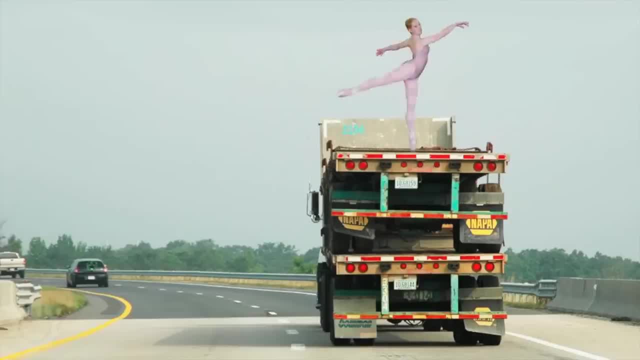 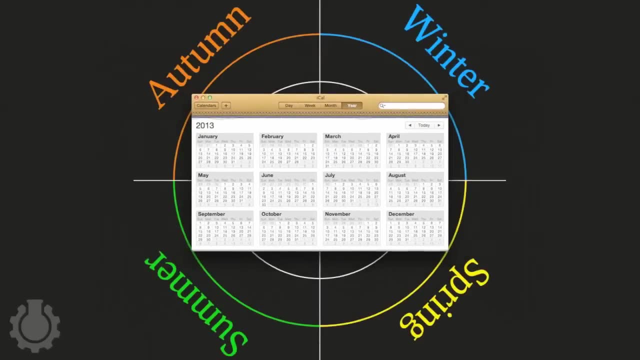 to the truck's cruising speed. Counting the number of ballerina turns to predict how long the truck takes to drive in a circle might give you a rough idea, but it's crazy to expect it to be precise. Counting the days to track the orbit is pretty much the same thing, and 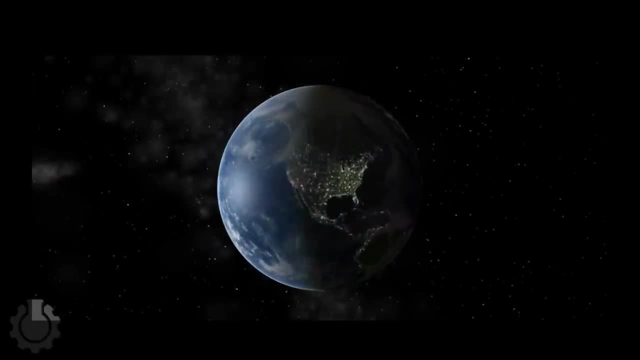 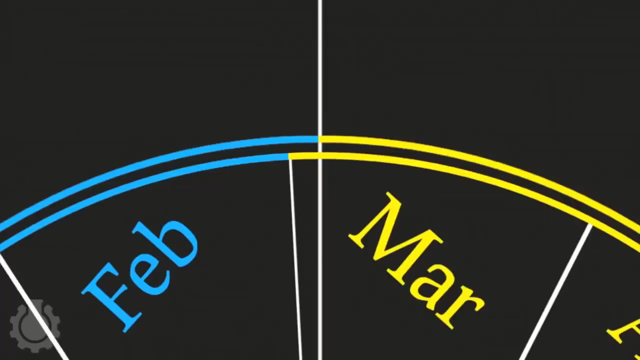 so it shouldn't be a surprise when the earth doesn't happen to make 365 complete spins in a year. Irritatingly, while 365 days are too few, 366 days are too many and still cause the seasons to drift out of sync just in the 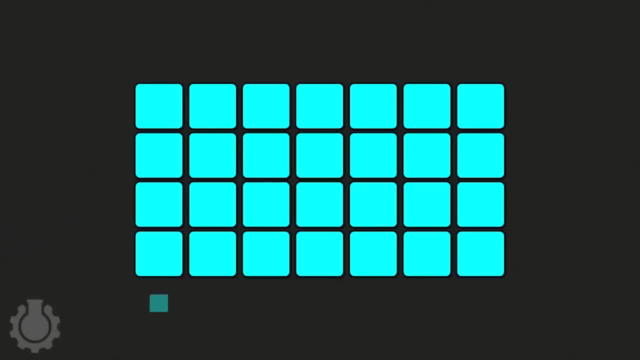 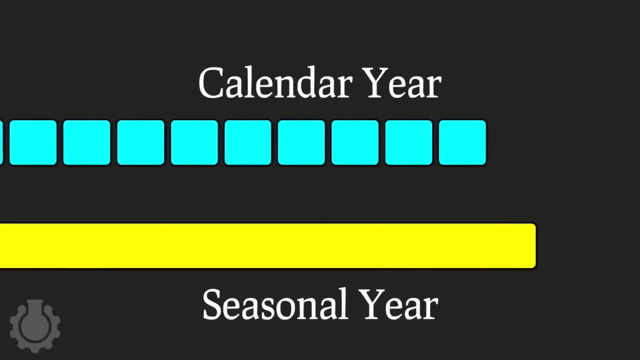 opposite way. The solution to all this is the leap year, where February gets an extra day, but only every 4 years. This works pretty well, as each year the calendar is about a quarter day short, so after 4 years you add an extra day to get back in alignment. Huzzah, the problem has. 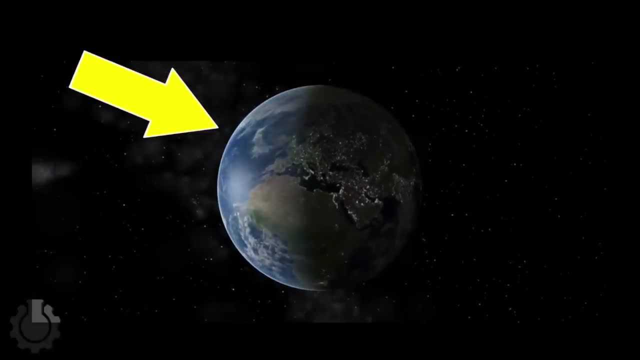 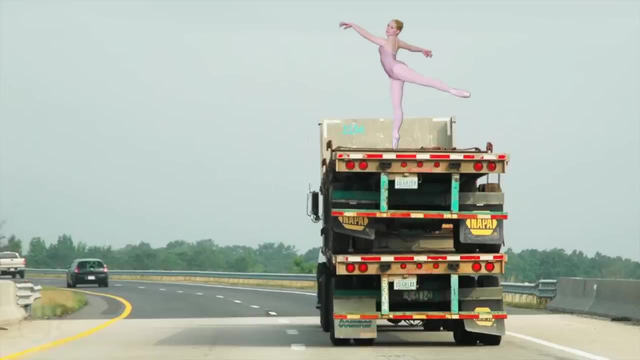 earth rotating about its axis. when you're on the side facing the sun, it's daytime and when you're on the other side it's night. But this rotation is no more connected to the orbital motion around the sun than a ballerina spinning on the back of a truck is connected. 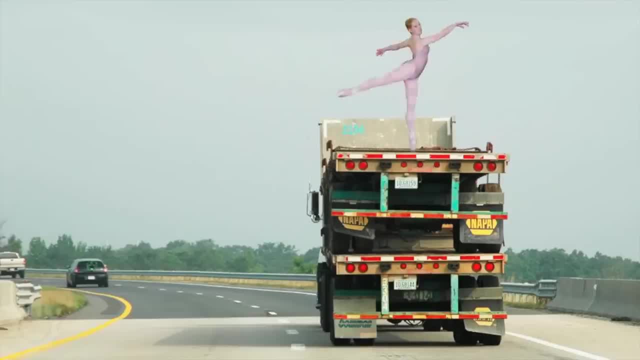 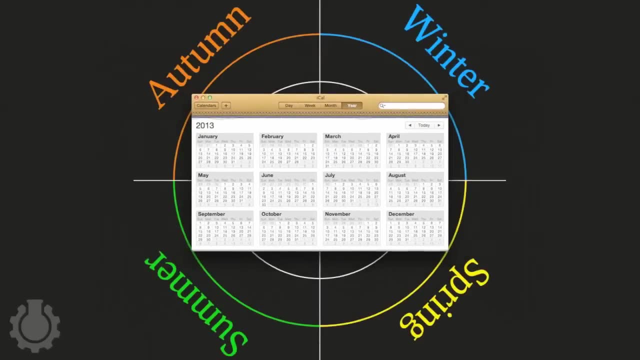 to the truck's cruising speed. Counting the number of ballerina turns to predict how long the truck takes to drive in a circle might give you a rough idea, but it's crazy to expect it to be precise. Counting the days to track the orbit is pretty much the same thing, and 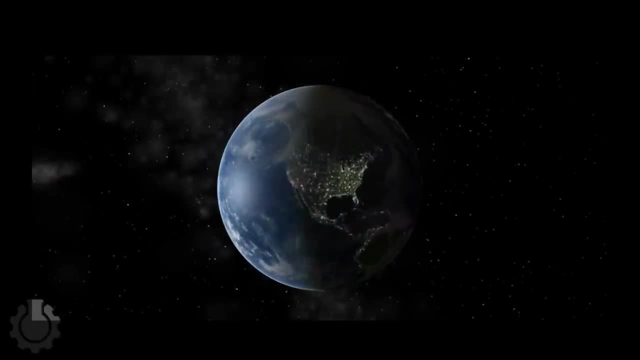 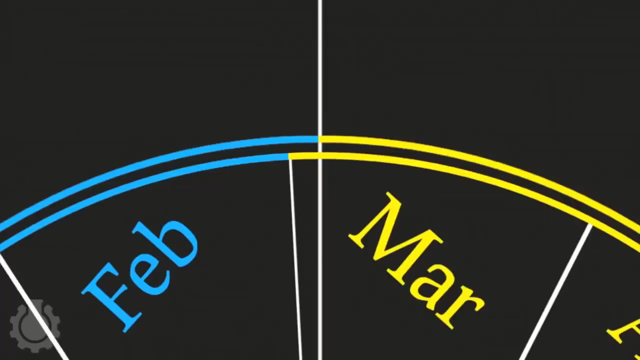 so it shouldn't be a surprise when the earth doesn't happen to make 365 complete spins in a year. Irritatingly, while 365 days are too few, 366 days are too many and still cause the seasons to drift out of sync just in the 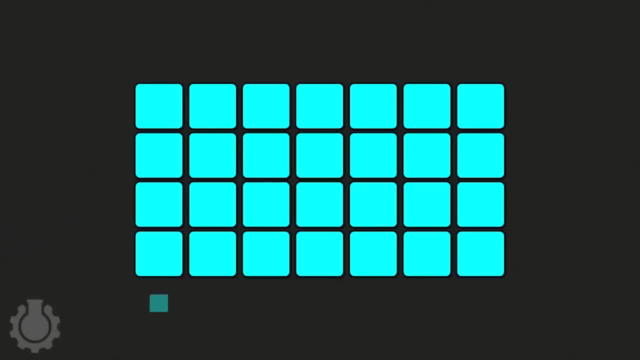 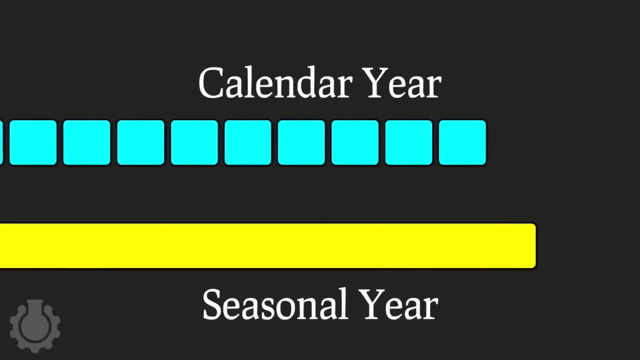 opposite way. The solution to all this is the leap year, where February gets an extra day, but only every 4 years. This works pretty well, as each year the calendar is about a quarter day short, so after 4 years you add an extra day to get back in alignment. Huzzah, the problem has. 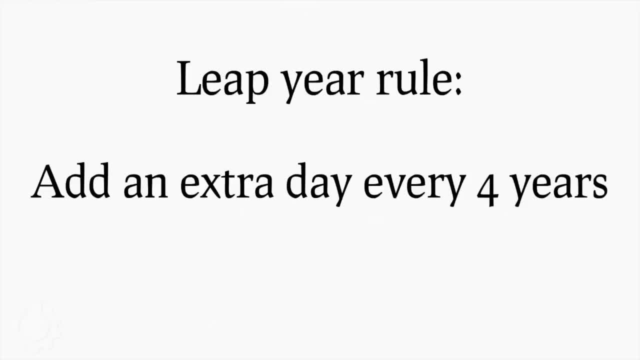 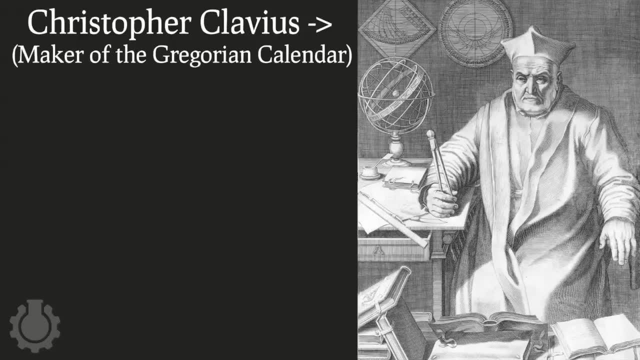 been solved, Except it hasn't. Lengthening the calendar by 1 day every 4 years is slightly too much, and the calendar still falls behind the seasons at a rate of 1 day per 100 years, which is fine for the apathetic, but not for calendar designers who want everything to. 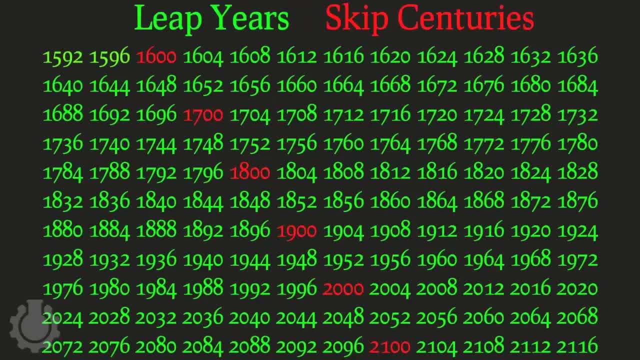 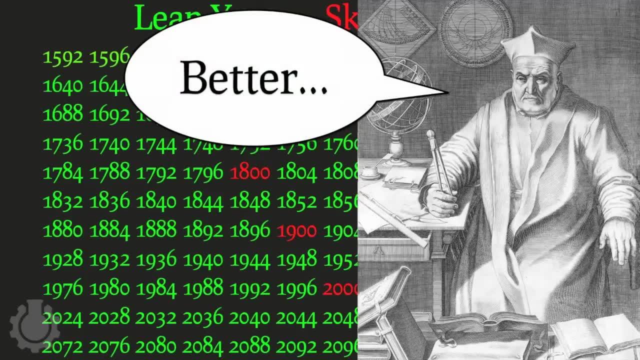 line up perfectly. To fix the irregularity, every century the leap year is skipped, so 1896 and 1904 were linked to the leap year. This is better, but still leaves the calendar ever so slightly too fast with an error of. 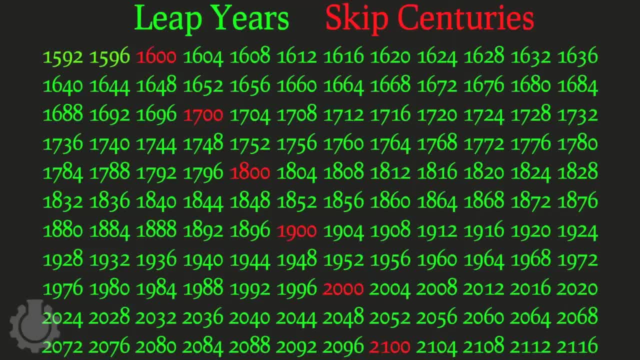 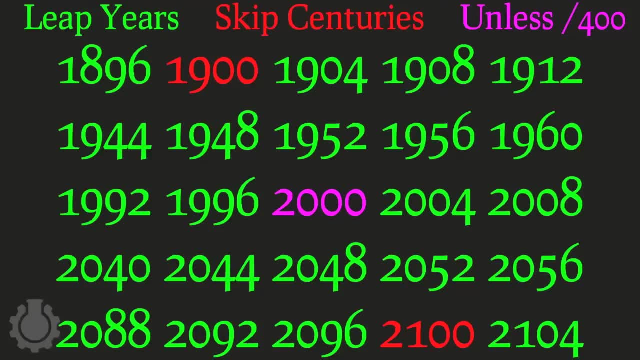 1 day in 400 years. so an additional clause is added to the skip the century rule that if the century is divisible by 400, then it will be a leap year. So 1900 and 2100 aren't leap years, but 2000 is. With these three rules, the error is now just 1 day off, and 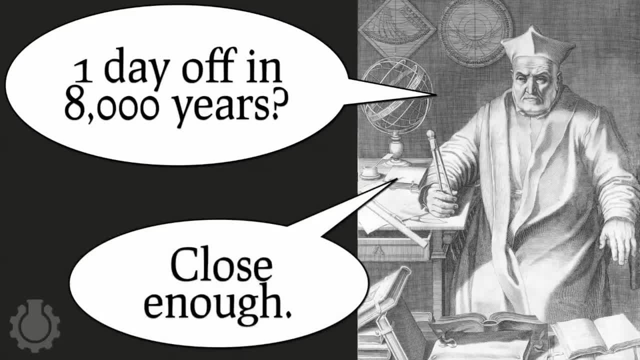 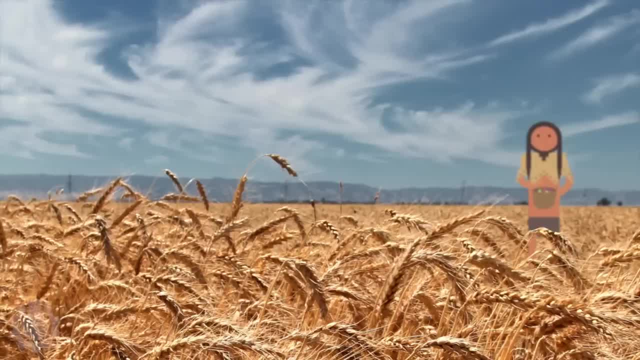 almost 8000 years which the current calendar declares mission accomplished and so calls it a day, Which is probably quite reasonable, because 8000 years ago humans were just figuring out that farming might be a good idea, and 8000 years from now we'll hopefully be using a calendar with a better date tracking. 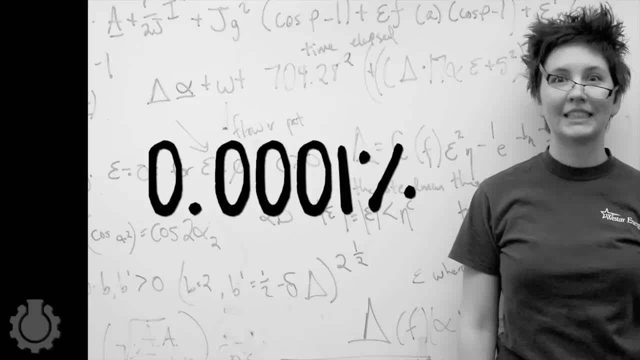 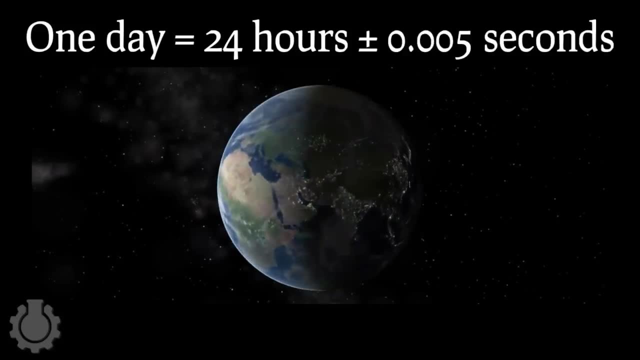 system. But perhaps you're a mathematician and a 0.0001% error is an abomination in your eyes and must be removed. Tough luck, says the universe, because the length of a day isn't even consistent. It randomly varies a few milliseconds on average and very slowly decreases. 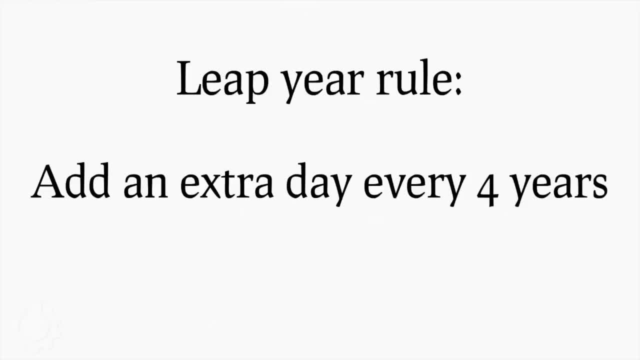 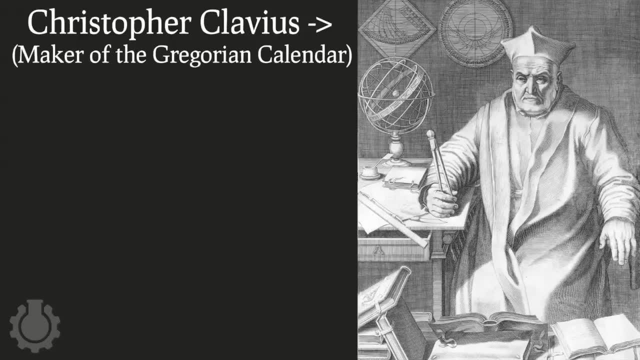 been solved, Except it hasn't. Lengthening the calendar by 1 day every 4 years is slightly too much, and the calendar still falls behind the seasons at a rate of 1 day per 100 years, which is fine for the apathetic, but not for calendar designers who want everything to. 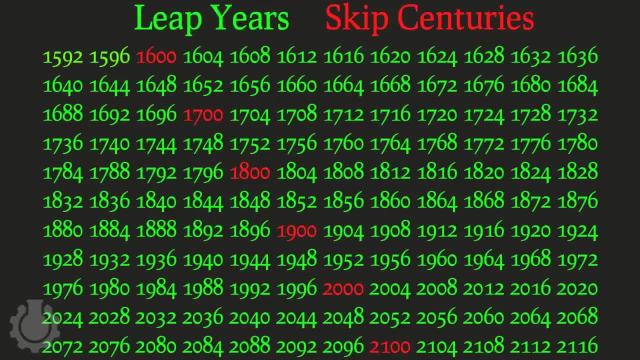 line up perfectly. To fix the irregularity, every century the leap year is skipped. so 1896 and 1904 were linked to the leap year. 1906 and 1904 were leap years, but 1900 wasn't. This is better but still leaves the calendar. 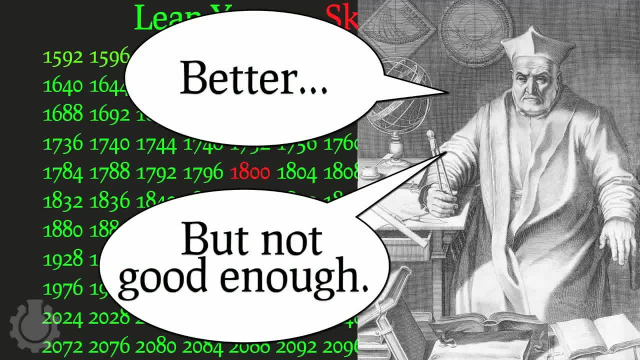 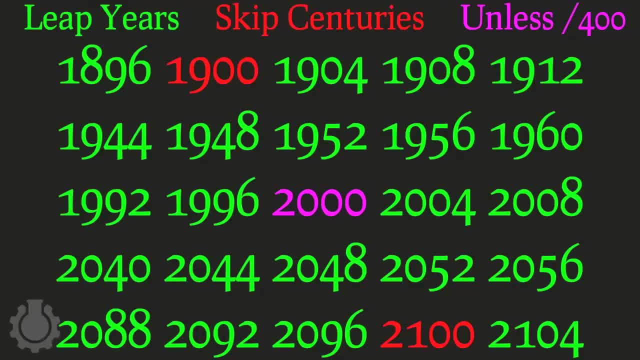 ever so slightly too fast, with an error of 1 day in 400 years. So an additional clause is added to the skip the century rule that if the century is divisible by 400, then it will be a leap year. So 1900 and 2100 aren't leap years, but 2000 is, With these three. 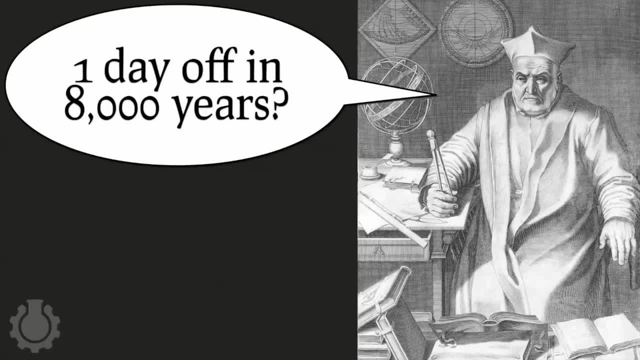 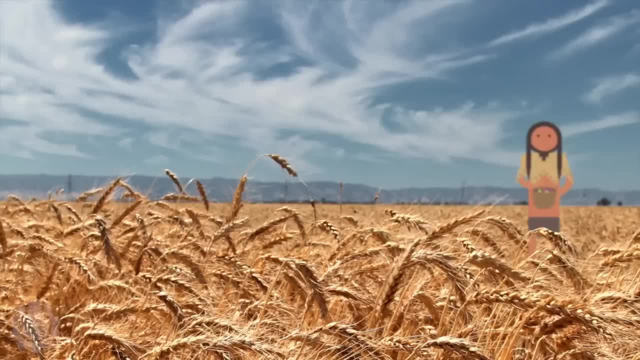 rules. the error is now just 1 day off and almost 8000 years, which the current calendar declares mission accomplished and so calls it a day, Which is probably quite reasonable, because 8000 years ago humans were just figuring out that farming might be a good idea and 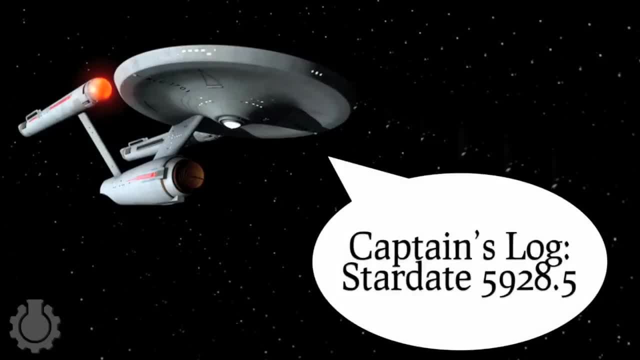 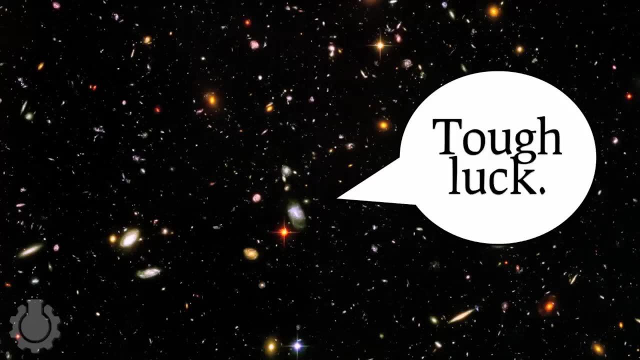 8000 years from now, we'll hopefully be using a calendar with a better date tracking system. But perhaps you're a mathematician and a 0.0001% error is an abomination in your eyes and must be removed. Tough luck, says the universe, because the length of a day isn't even consistent. It randomly varies a few milliseconds on average and very slowly decreases by about 1 millisecond per 100 years, which means it's literally impossible to build a perfect calendar that lasts forever. In theory, the length of a day will expand to be as long as the current month. 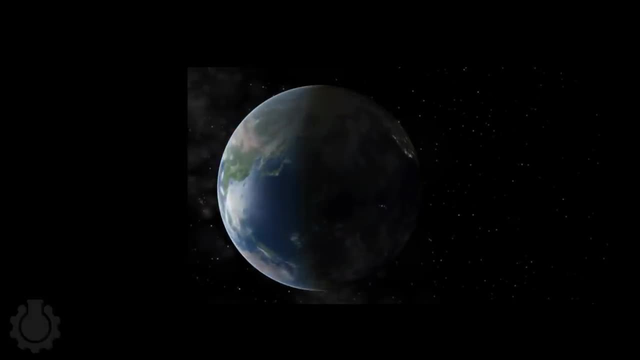 but don't worry. in practice it will take tens of billions of years and our own expanding sun will destroy the earth forever. That's why the calendar is called the calendar of the earth, long before that happens. Sorry, not quite sure how we got from counting the days of the months to the fiery unavoidable. end of all human civilization, unless, of course, we have an adequately funded space program. hint, hint, but there you have it. For the next 8 millennia, leap years will keep the calendar in sync with the seasons, but in a surprisingly complicated way. Thanks for watching and I'll see you in the next video. 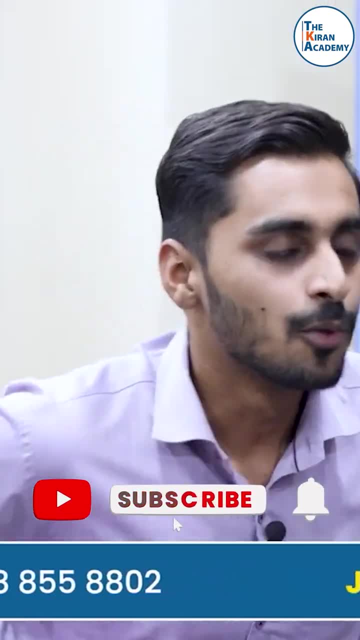 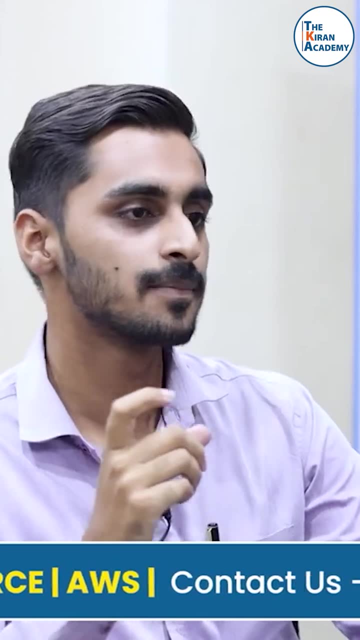 Explain OOPS concept in Java. Okay, OOPS concept. basically there are four pillars of OOPS concept and includes six, That is, class, object, encapsulation, polymorphism, abstraction and inheritance. Actually, coming to the encapsulation, encapsulation is the first pillar of OOPS. 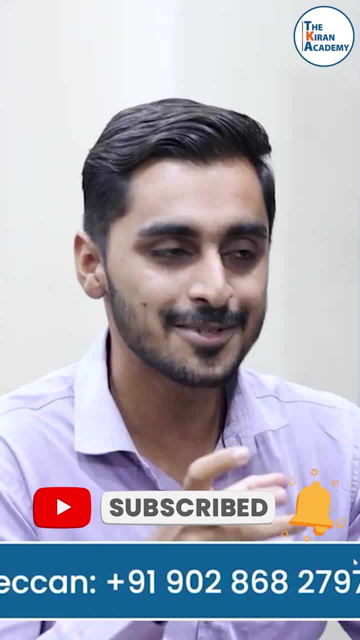 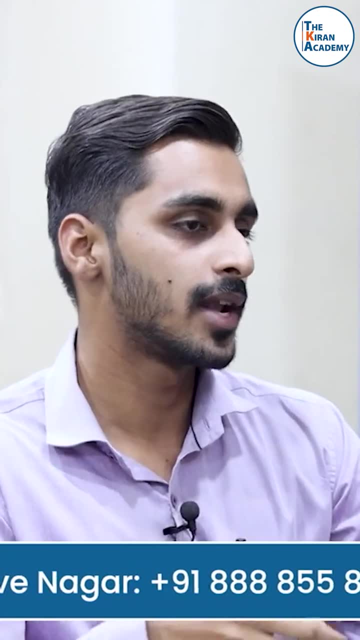 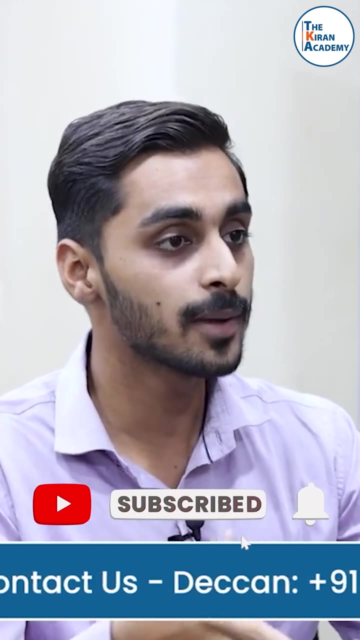 Encapsulation is the binding of related data. The main objective of encapsulation is data security And the best practice to do encapsulation is that: making global variable as private and accessing that global variables via public methods, via getter, setter methods. We can make private our ATM pin. So that's the encapsulation. by about 1 millisecond per 100 years, which means it's literally impossible to build a perfect calendar that lasts forever. In theory, the length of a day will expand to be as long as the current month, but don't worry, in practice it will take tens of billions. 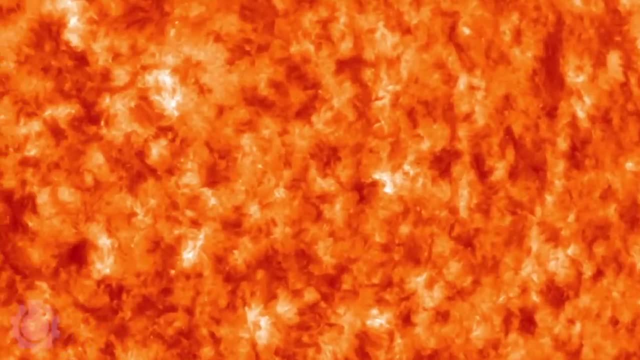 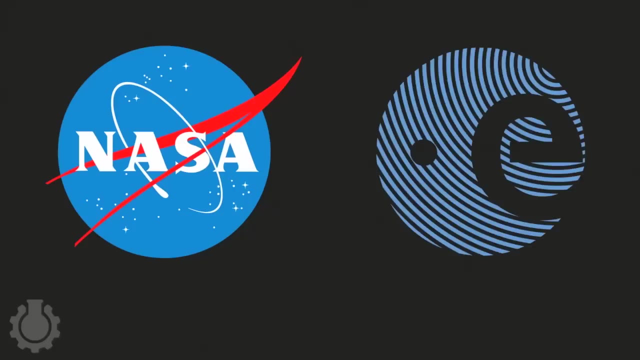 of years and our own expanding sun will destroy the earth forever. This is just one of the things that can happen. Sorry, not quite sure how we got from counting the days of the months to the fiery, unavoidable end of all human civilization, unless, of course, we have an adequately funded space program.